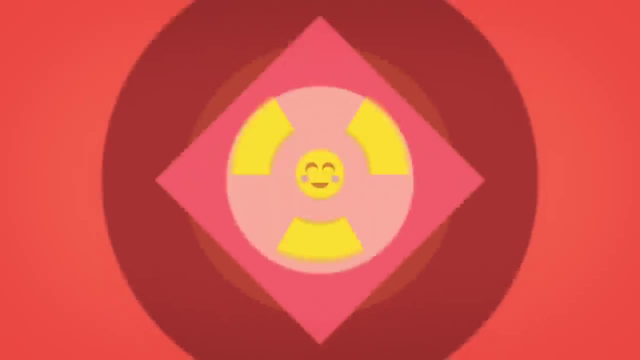 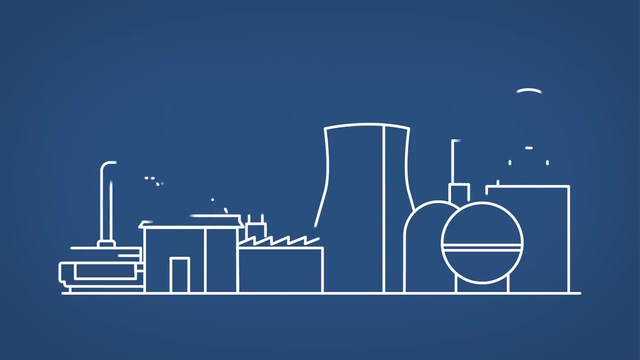 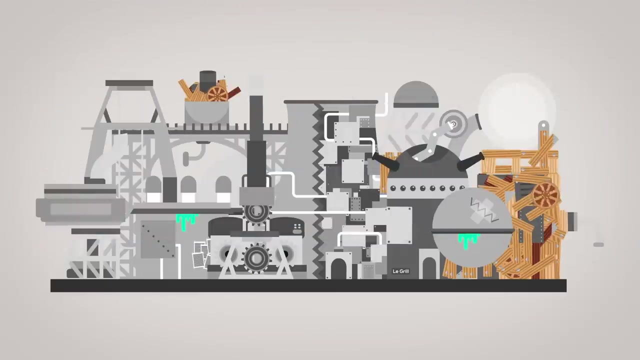 hard work away. One thing was certain: the future was atomic. Just a few years later there was a sort of atomic age hangover. As it turned out, nuclear power was very complicated and very expensive. Turning physics into engineering was easy on paper but hard in. 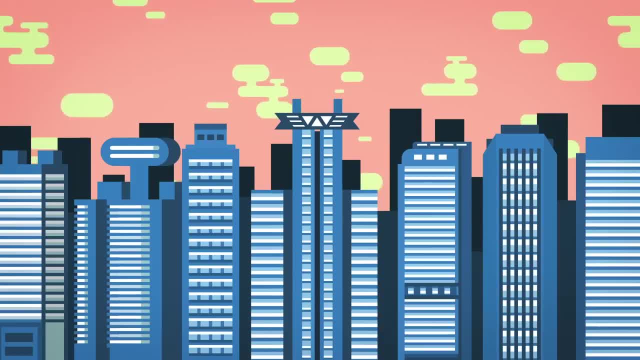 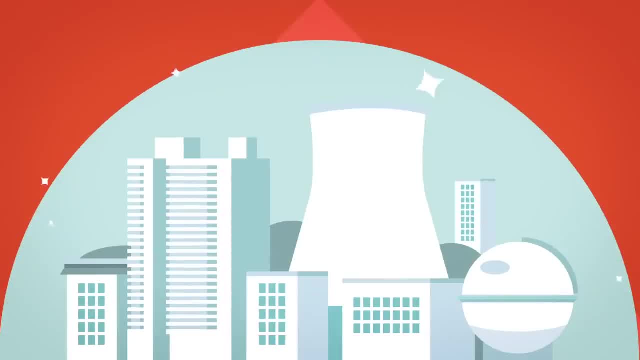 real life. Also, private companies thought that nuclear power was much too risky as an investment. Most of them would much rather stick with gas, coal and oil. But there were many people who didn't just want to abandon the promise of the atomic age, An exciting new technology. 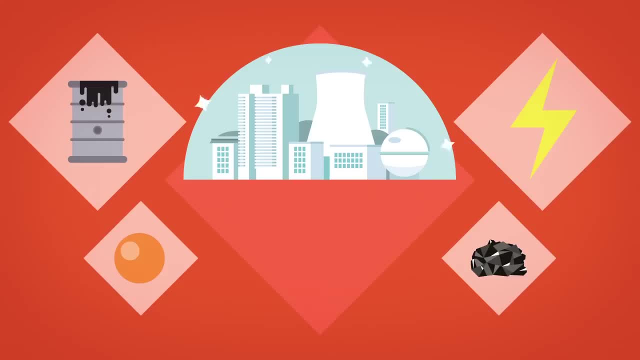 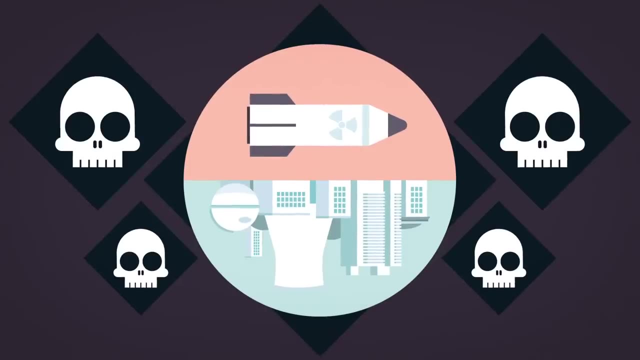 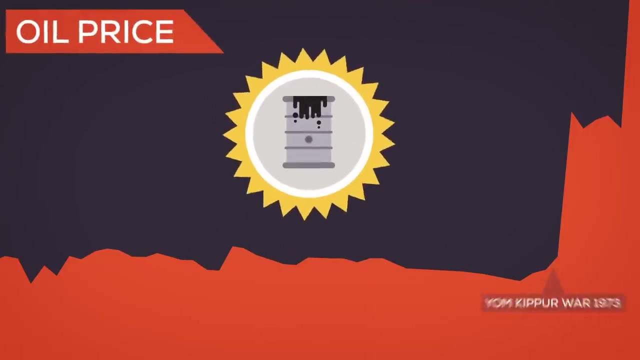 the prospect of enormously cheap electricity, the prospect of being independent of oil and gas imports and, in some cases, a secret desire to possess atomic weapons, provided a strong motivation to keep going. Nuclear power's finest hour, the first of its kind, was the early 1970s, when war in the Middle East caused oil prices. to skyrocket worldwide. Now commercial interest and investment picked up at a dazzling pace. More than half of all the nuclear reactors in the world were built between 1970 and 1985.. But which type of reactor to build, given how many different types there were to choose? 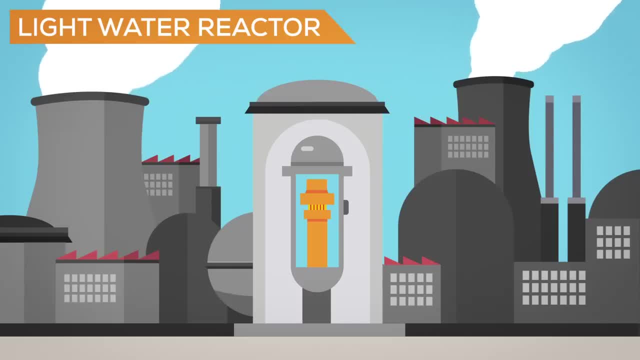 from A surprising underdog candidate won the day: the light water reactor. It wasn't very innovative and it wasn't too popular with scientists, but it was a very popular reactor. It was the first reactor to be built in the world. It was the first reactor to 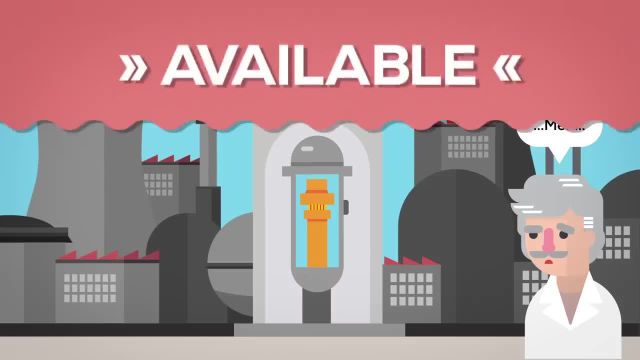 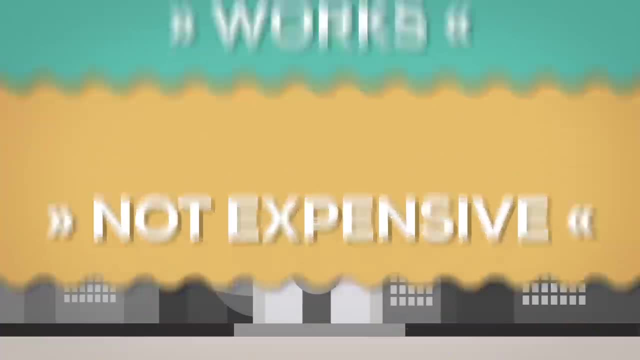 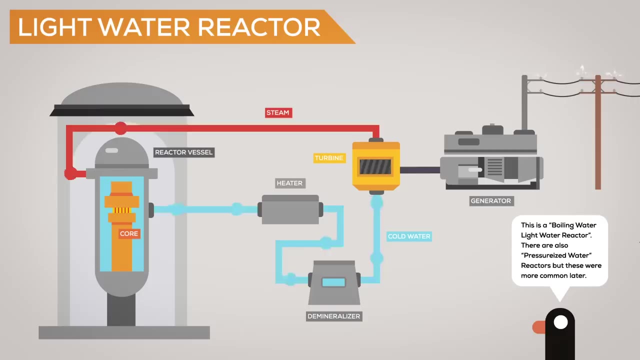 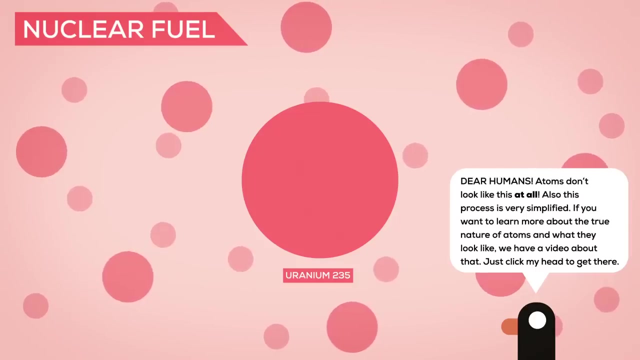 was there, it worked and it wasn't terribly expensive. So what does a light water reactor do? Well, the basic principle is shockingly simple. It heats up water using an artificial chain reaction. Nuclear fission releases several millions times more energy than any chemical reaction could Really heavy elements on the 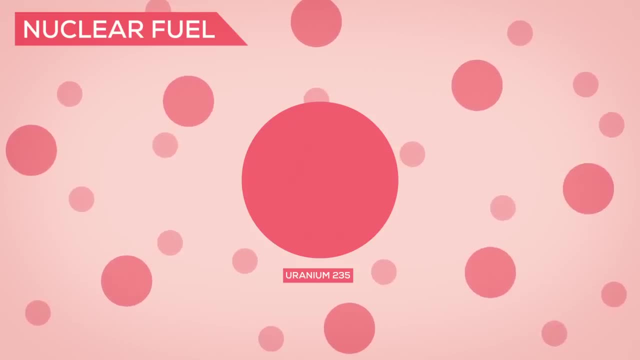 brink of stability, like uranium 235, get bombarded with neutrons. The neutron is absorbed, but the result is unstable Most of the time. it immediately splits into fast-moving lighter elements, some additional free neutrons and energy in the form of radiation. 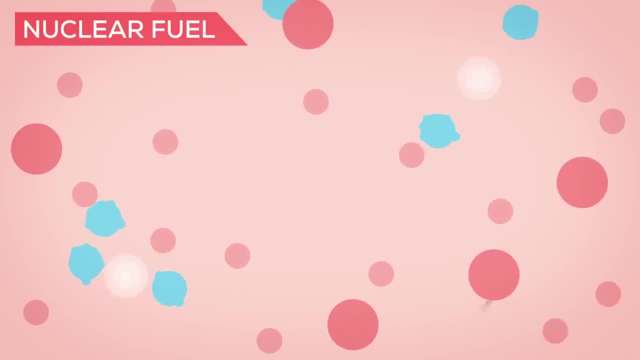 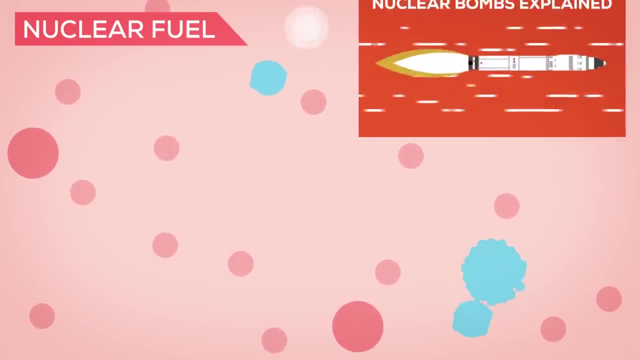 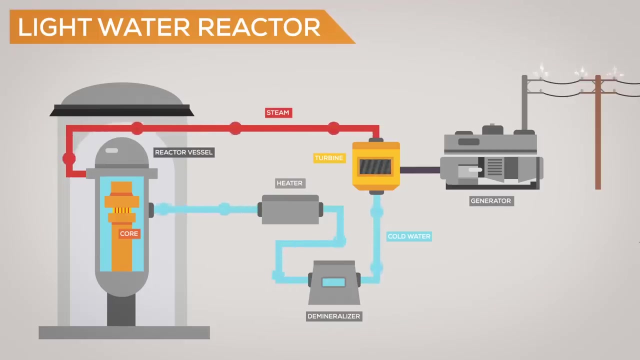 The radiation heats the surrounding water, while the neutrons repeat the process with other atoms releasing more neutrons and radiation in a closely controlled chain reaction, Very different from the fast, destructive runaway reaction in an atomic bomb. In our light water reactor, a moderator is needed to control the neutron's energy.